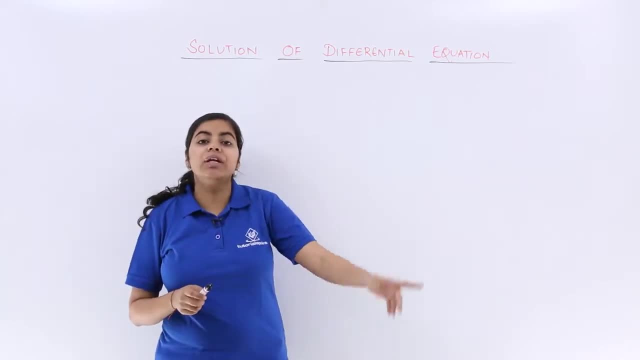 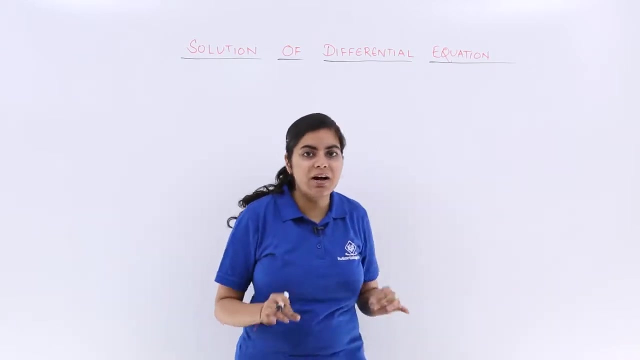 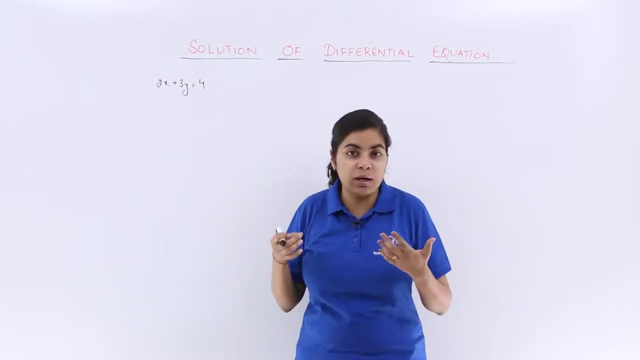 So linear and quadratic equations we have studied. We have also studied how to compute the solution. A linear equation is there, You know how to compute its solution. You know similarly about the quadratic equation. Let me tell you with an example. I know that I have a linear equation. say 2x plus 3y is equal to say 4.. Very randomly I have written: This is a linear equation in two variables, x and y. How did we get about the solution? We saw that there are two variables, So we need one more equation. Suppose there is another equation. You either use elimination or elimination. 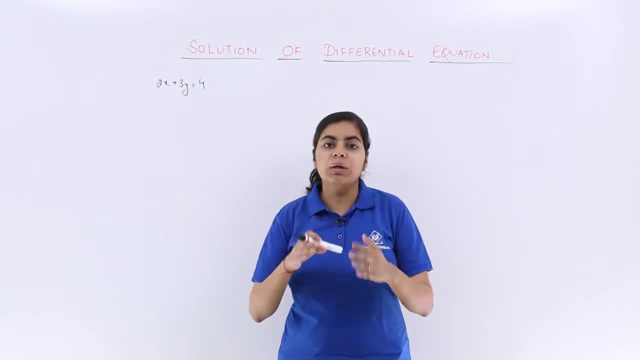 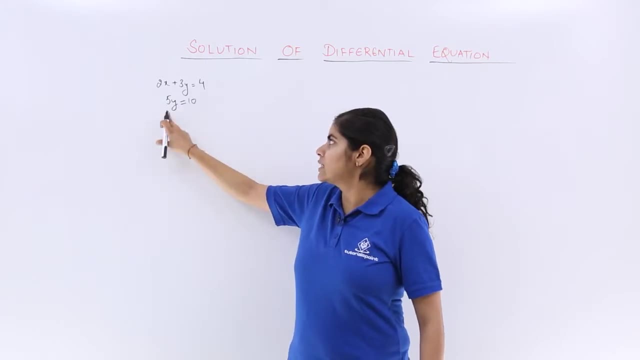 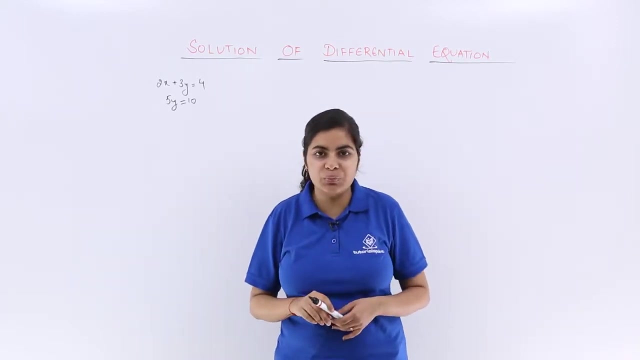 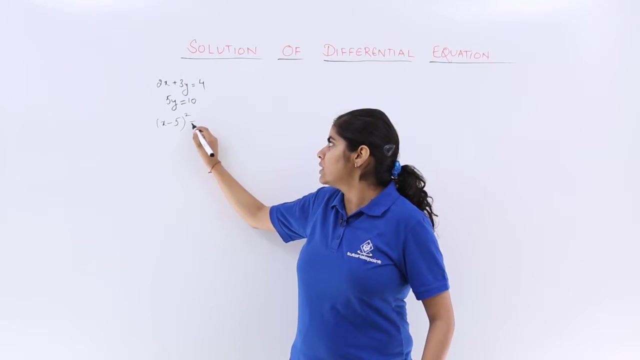 You either use elimination method or you use substitution method and so on. But what about a quadratic equation and what about something of this sort? Say I have 5y is equal to 10.. This is another equation, Linear equation, in only one variable. What is the value of y? y is equal to 10 upon 5, which is 2.. Similarly, if you have x minus, say 5, whole square is equal to say 0.. So how do you get the solution for this? You can find out by looking at the equation. 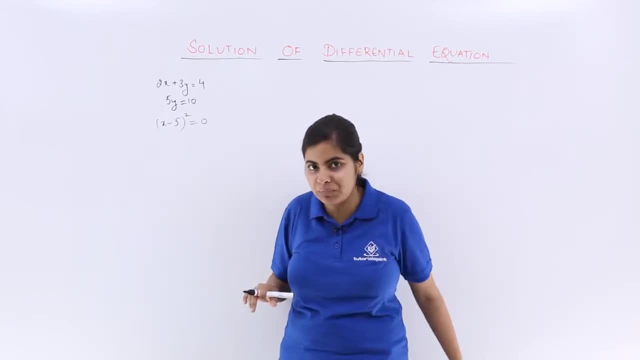 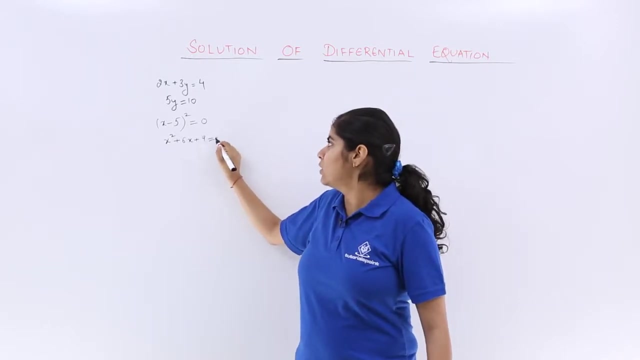 You know how to compute it. This is a quadratic equation in one variable. Next, let us see if I have x square, say plus 6x plus any other thing can be there, right- Plus 9 is equal to 0.. So this is the formula of x plus 3, whole square. 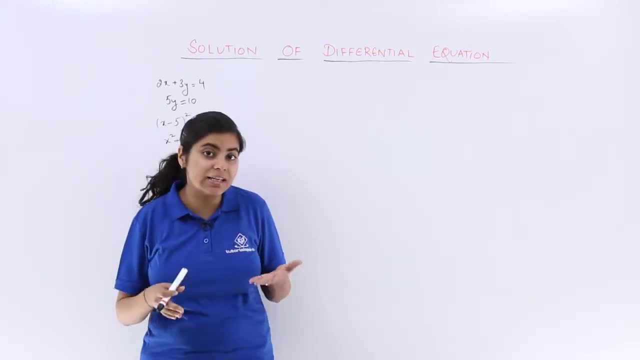 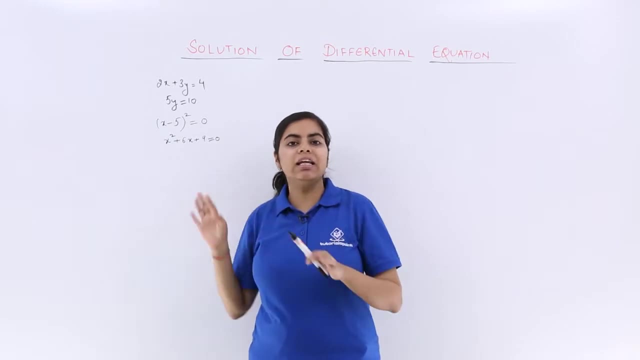 So when you have different equations, you know how to solve them and get a solution. And what is meant by solution? What value, when you put in this equation, will make it equal to the right hand side. That is solution. So left hand side. 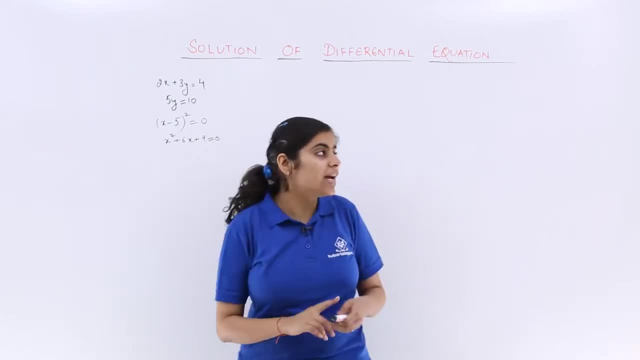 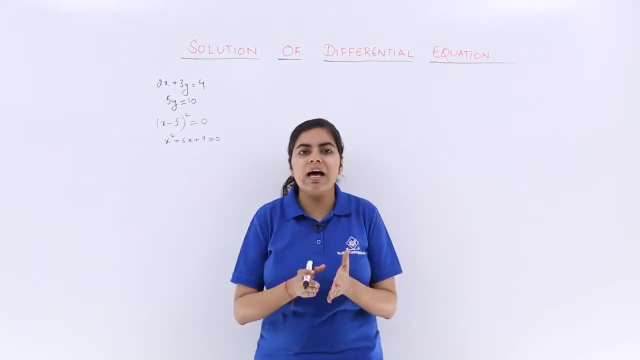 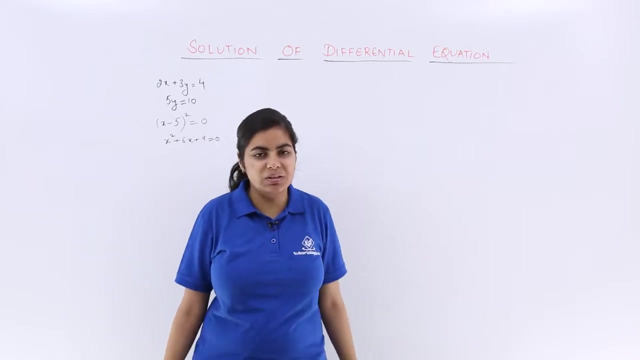 should be equal to right hand side. That is known as the solution. And what about the case of differential equation solution? So differential equation solution means you must have something in your back of your mind so that again the left hand side and the right hand side becomes equal.